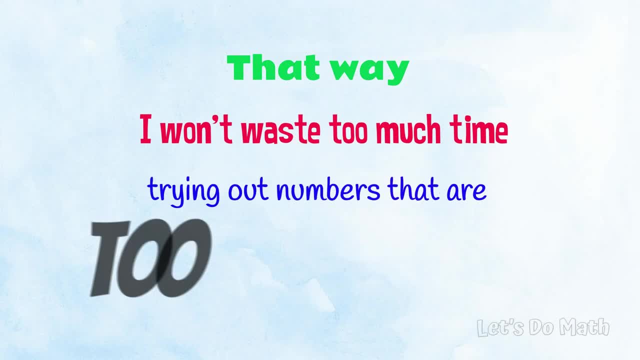 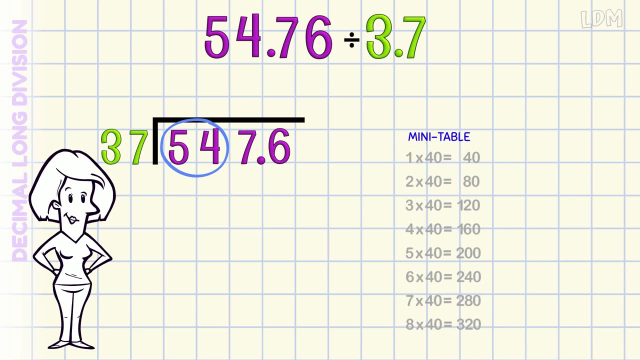 That way I won't waste too much time trying out numbers that are too low or too high. Now let's divide How many 37s in 54? There's only one. Put 37 under 54 and now we subtract to find the remainder. 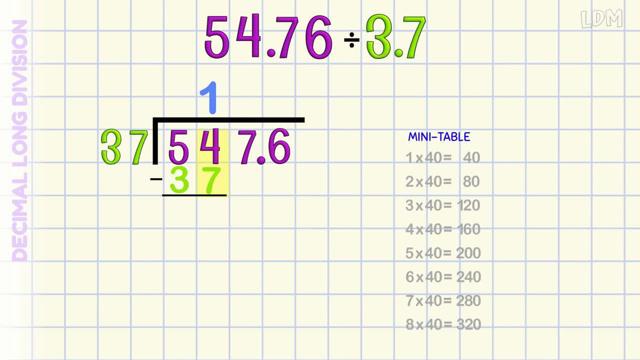 4 minus 7?? Can't do it, I need to borrow a 10. 5? 5 becomes 4, and there's the 10 I borrowed. Now we have 14 minus 7.. That's 7.. And 4 minus 3 is 1.. 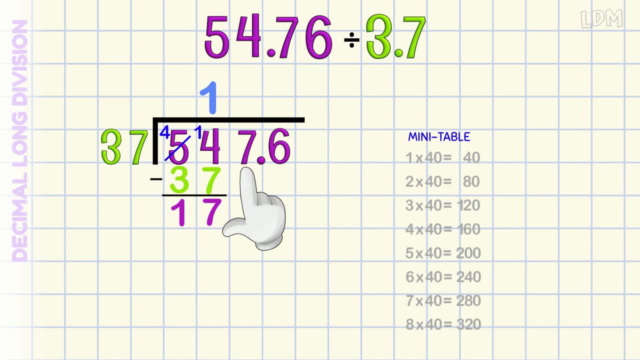 The remainder is 17.. Bring down the next digit to make the next number. we consider How many 37s in 177?? My mini-table for 40 tells me that 4 is the number to choose. Set up 37 times 4.. 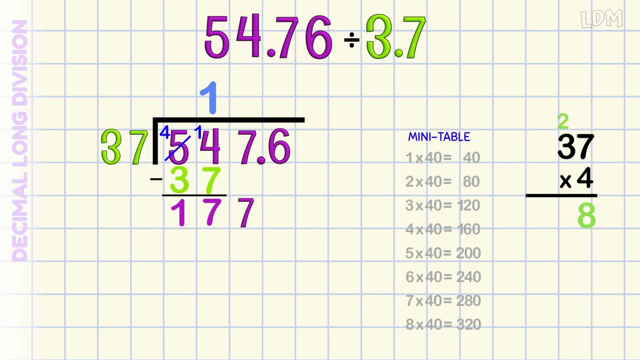 4 times 7 is 28? And 4: 3s are 12.. Plus 2 is 14.. Do I need to go to 37 times 5?? I can test that. Just adding another 30 gets me to 178.. 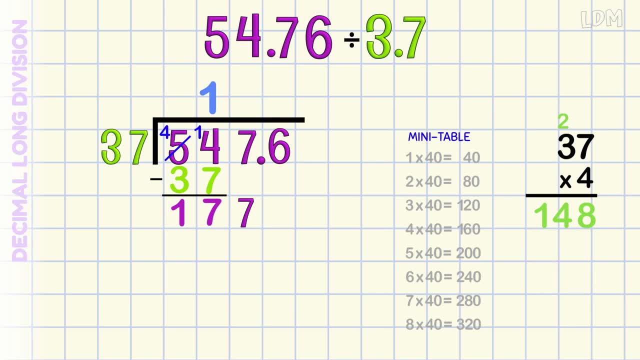 Too much, So I know that 4 is a fit. I put 4 on the answer line and a decimal point matching the one in the dividend. 148 goes here, ready to find the remainder. Now we subtract 7 minus 8?. 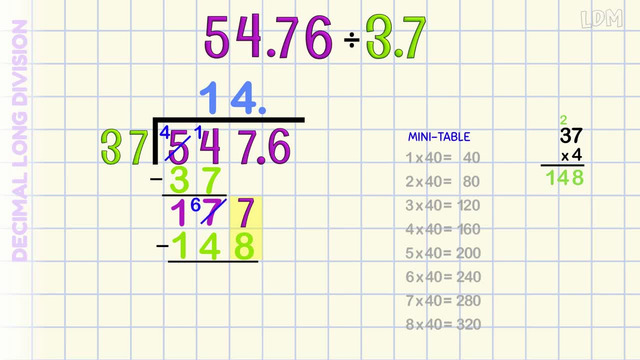 Can't do it, I need to borrow a 10.. 7 becomes 6, and there's the 10 I borrowed. Now we have 17 minus 8.. Well, 18 minus 8 would be 10.. This is 1 less, so it's 9.. 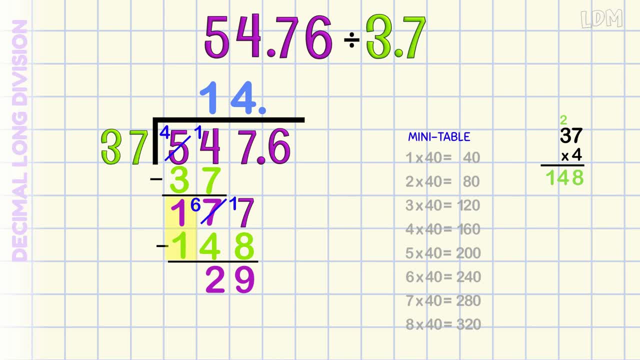 Now 6 minus 4 is 2, and these ones just cancel out. Last step: Bring down the 6.. My final question is: how many 37s in 296?? That's a big one. That's why I need a mini-table. 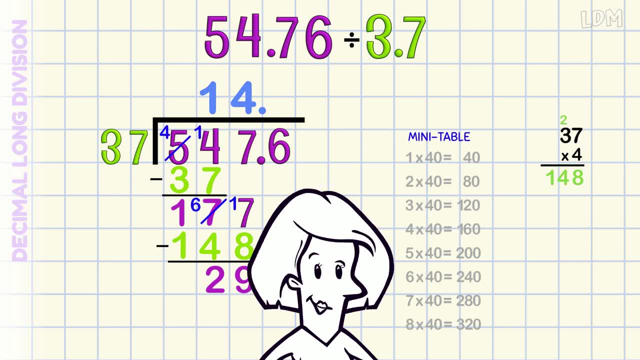 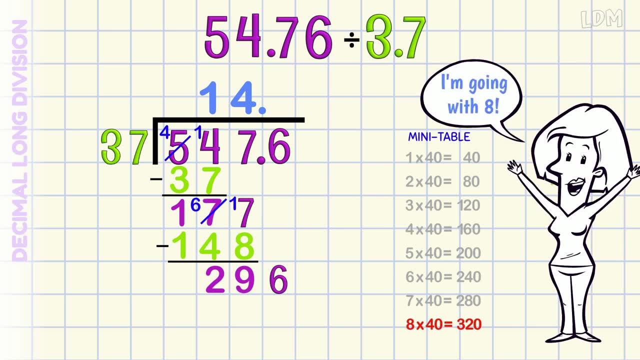 to help gauge exactly which value to try: 8 times 40 is 320.. It's a bit high, but this mini-table is rounded up. I'm going with 8.. Let's multiply: 7 times 8 is 56. 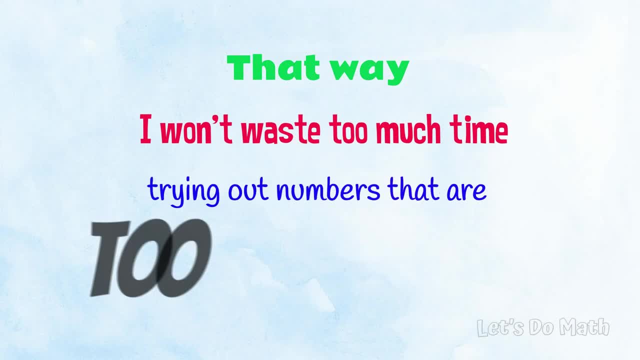 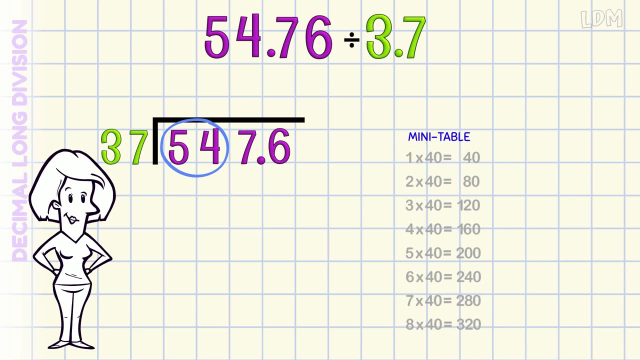 That way I won't waste too much time trying out numbers that are too low or too high. Now let's divide How many 37s in 54? There's only one. Put 37 under 54 and now we subtract to find the remainder. 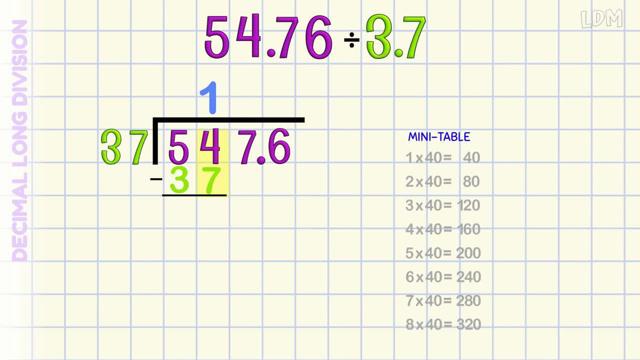 4 minus 7?? Can't do it, I need to borrow a 10. 5? 5 becomes 4, and there's the 10 I borrowed. Now we have 14 minus 7.. That's 7.. And 4 minus 3 is 1.. 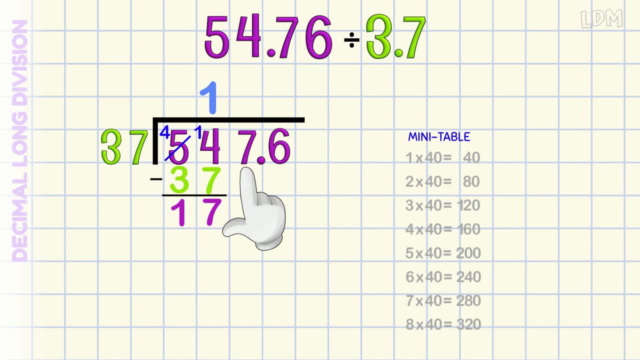 The remainder is 17.. Bring down the next digit to make the next number. we consider How many 37s in 177?? My mini-table for 40 tells me that 4 is the number to choose. Set up 37 times 4.. 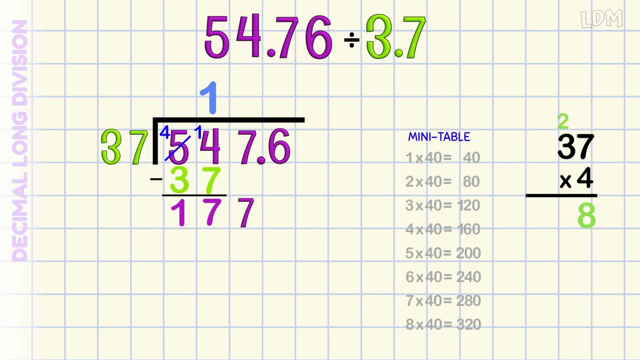 4 times 7 is 28? And 4: 3s are 12.. Plus 2 is 14.. Do I need to go to 37 times 5?? I can test that. Just adding another 30 gets me to 178.. 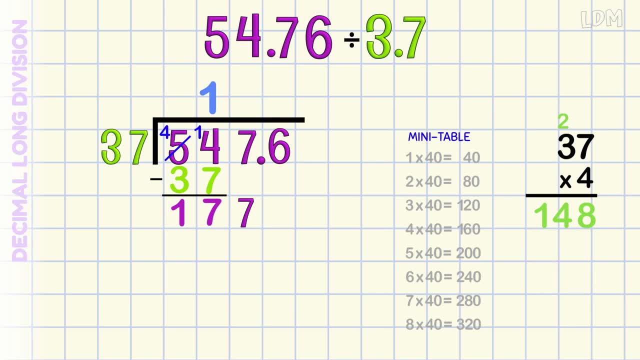 Too much, So I know that 4 is a fit. I put 4 on the answer line and a decimal point matching the one in the dividend. 148 goes here, ready to find the remainder. Now we subtract 7 minus 8?. 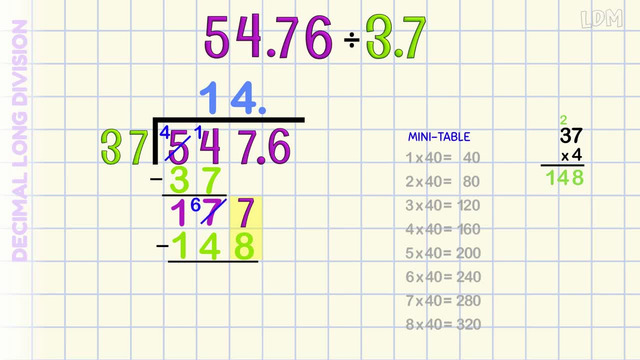 Can't do it, I need to borrow a 10.. 7 becomes 6, and there's the 10 I borrowed. Now we have 17 minus 8.. Well, 18 minus 8 would be 10.. This is 1 less, so it's 9.. 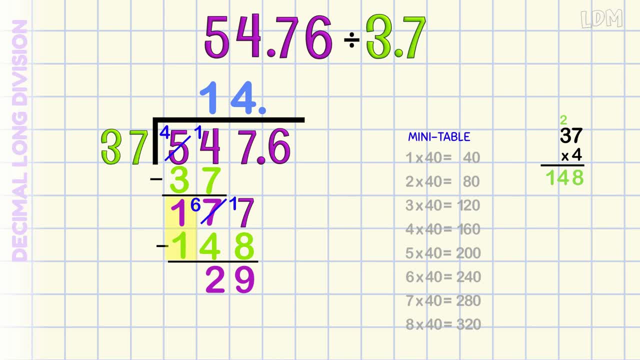 Now 6 minus 4 is 2, and these ones just cancel out. Last step: Bring down the 6.. My final question is: how many 37s in 296?? That's a big one. That's why I need a mini-table. 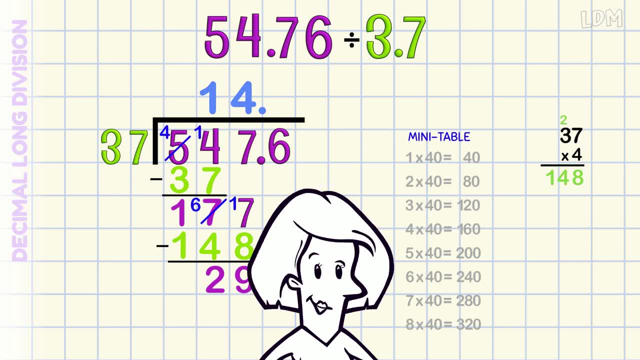 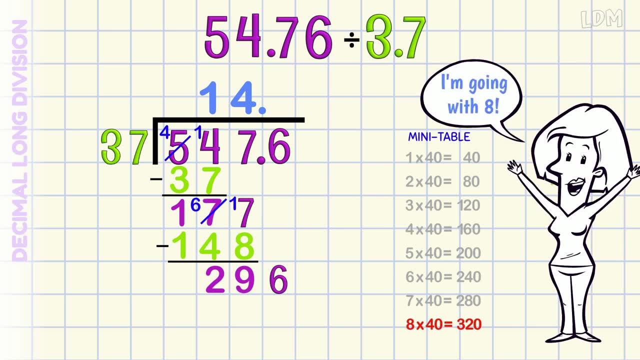 to help gauge exactly which value to try: 8 times 40 is 320.. It's a bit high, but this mini-table is rounded up. I'm going with 8.. Let's multiply: 7 times 8 is 56.